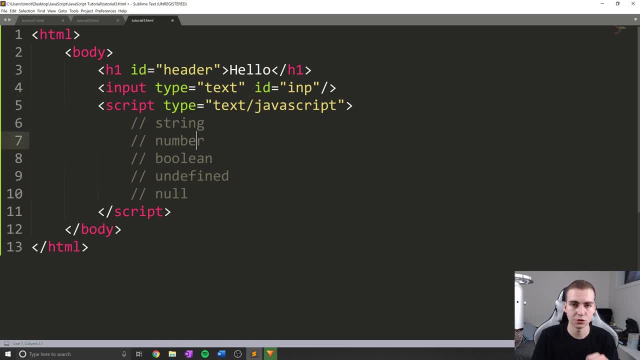 we have no, And these are the five primitive Java data types. So let's add that here. Prim it to vice, definitely, prim it to butcher that word. Anyways, there we go. Okay, primitive, So what is a string? We'll do it, actually, before the comment. 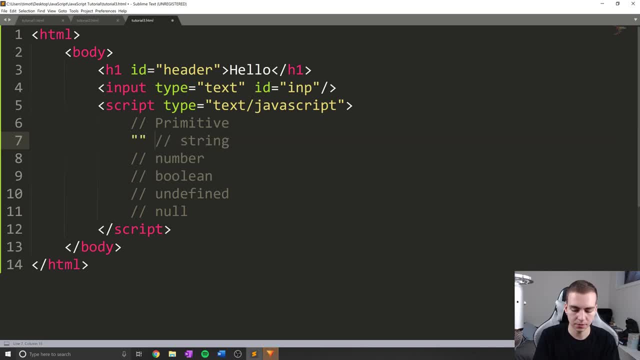 A string is essentially anything inside of double or single quotation marks, And that is all that a string is Essentially. the rule for string is: if it's inside of quotation marks- double or single- it is a string. doesn't matter what's inside of it. If it's inside of there, it is a string. And 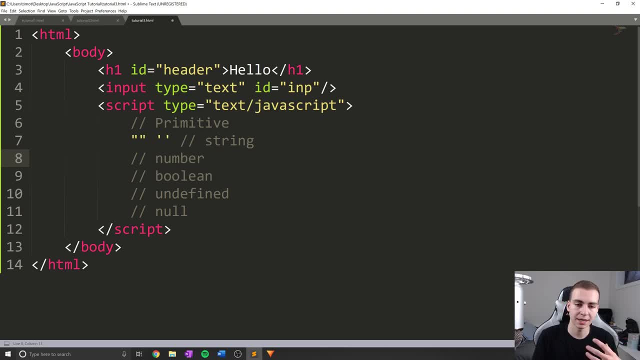 that is the only thing you need to know to remember strings. Now, a string is a kind of collection of characters. So if I do something like this, this is a string and the value is Hello. if I do something like 23.. This is a 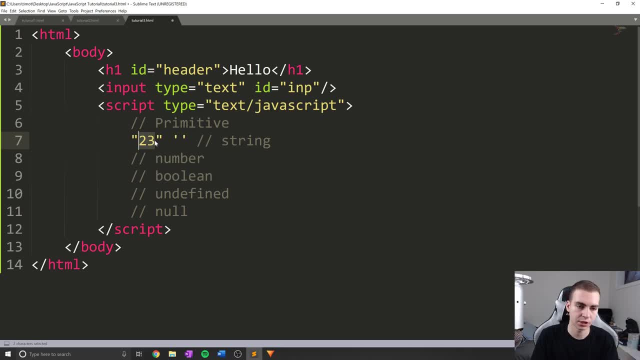 string. the value is 23.. Why is it a string? because it's inside quotation marks. that's all you need to know. collection of characters. I can do, random characters, I can do, you know, anything I want inside these quotation marks. Okay, number, what is a number? Well, that's. 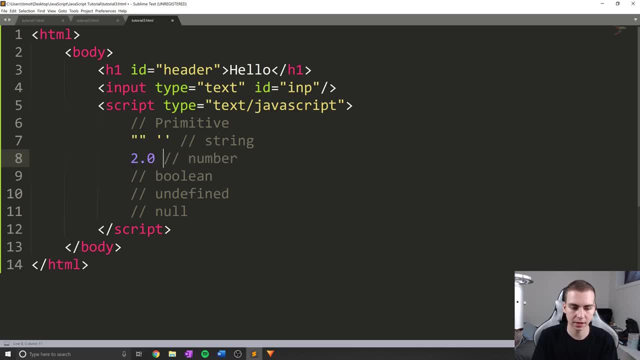 pretty straightforward. It is literally a number. So anytime we see something like 2.0, 8.99, negative 98, 1000, 0.000009.. These are all numbers, And notice that they highlight in purple and that they're not inside of quotation marks. So that is what a number is. But as 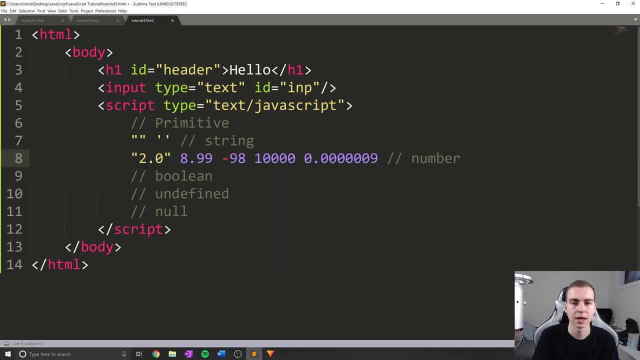 soon as I decide to put quotation marks around any of my numbers, they immediately become a string: Awesome. Now, just in case you see in other languages, I'm just going to let you know that if you do something that doesn't have a decimal point, that's typically referred. 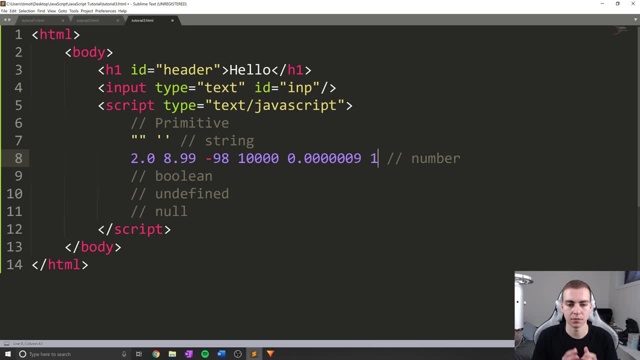 to as an integer, And an integer is anything that is, you know, doesn't have a floating decimal point representation, Whereas if I do something like 1.0, this is now what we call a string. So if I do something like 1.0, this is now what we call a string. So if I 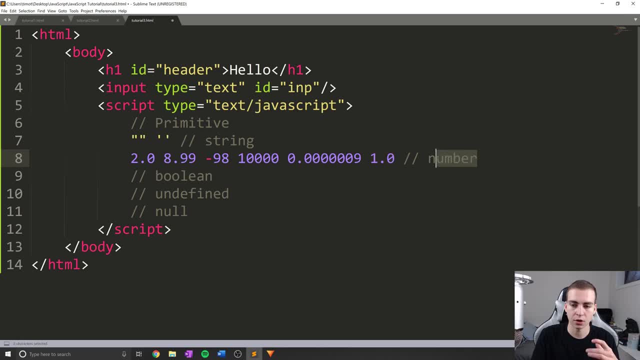 do something like 1.0, this is now what we call a float or a double. Now, this isn't important for Java, because these are all classified under the name number- sorry, JavaScript, But for other languages you might hear that. So I feel like I shouldn't have mentioned. 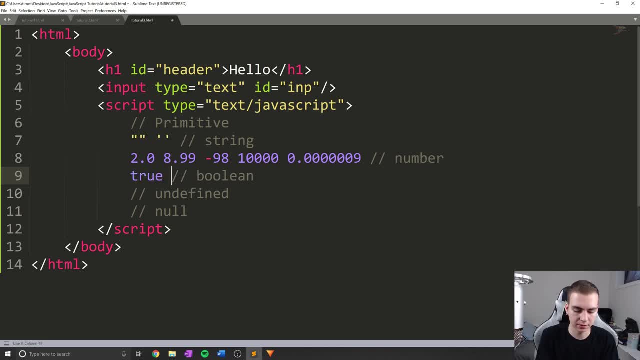 that to you guys. Okay, Boolean, this one's pretty easy. This is literally the values: true or false. So, Boolean just simply stands for true or false. you can either have true or you can either have false. there's no other values that fit into this category other than 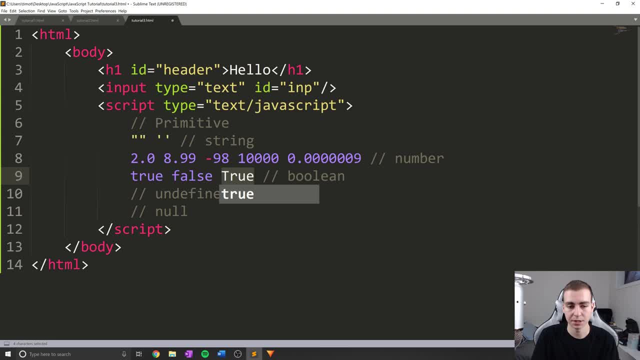 those two And notice that when I do true with a capital T, that is not the same as true with a lowercase t. So these two words, exactly the two words I've typed here, are the only values that are considered Boolean, And we'll talk about those later and why we use them undefined. Now. 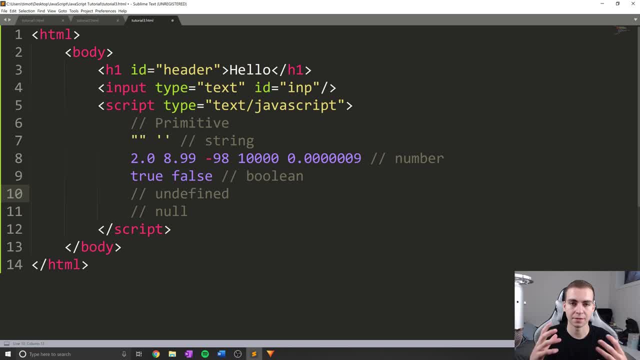 I'm not going to type anything here. The reason for that is because undefined simply means that we haven't defined something yet, And it's actually a type of its own. you can't really set a value to be undefined. it becomes undefined if you don't give it a value, And 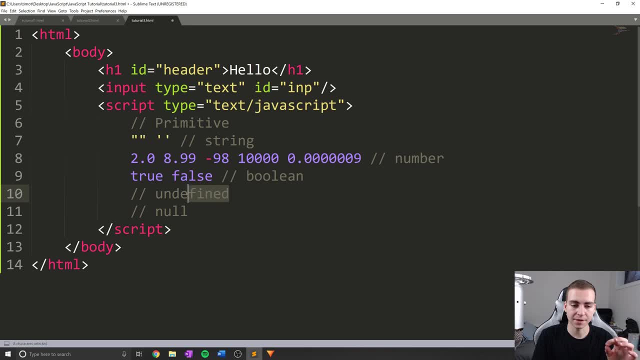 we'll understand that when we go into variables. Now, no is very similar to undefined, except it's actually a set value. So no means, you know, we're not storing anything yet. It's almost like, hey, we've set up kind of this empty container. we want to put something. 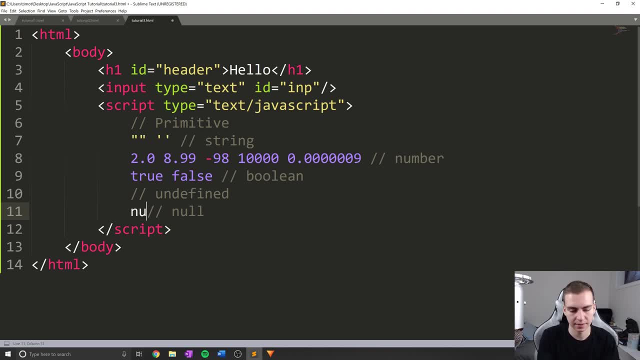 there, just so. like you know, it's okay, we have something, but it doesn't mean anything, And that's what no is. So when you type the word no, that's the type itself. That's all. that's considered No, And we'll talk about the difference between no and undefined later. 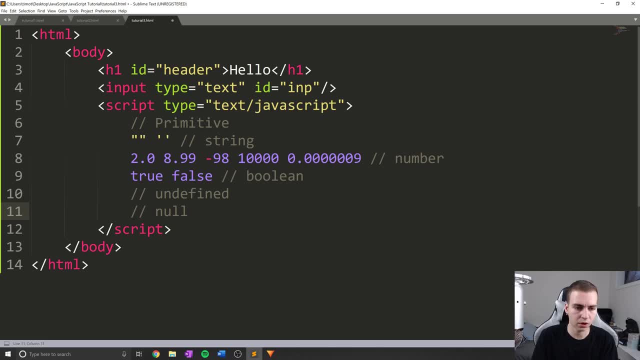 But they are very similar in nature. Okay, so those are our Java data types. Now I'm going to get rid of them And we're gonna start talking about variables. So we're going to talk about variables. So variables are capable of storing any kind of data type. 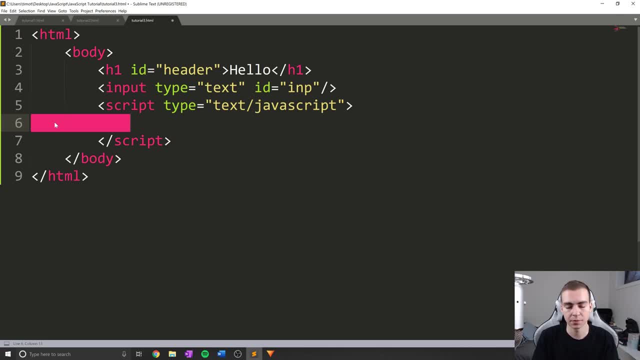 Now that could be a primitive data type or it could be a reference data. Again, you don't need to know the difference, but a variable is capable of storing some value. Now, the way that we define a variable inside of Java was a few different ways, or sorry, I keep. 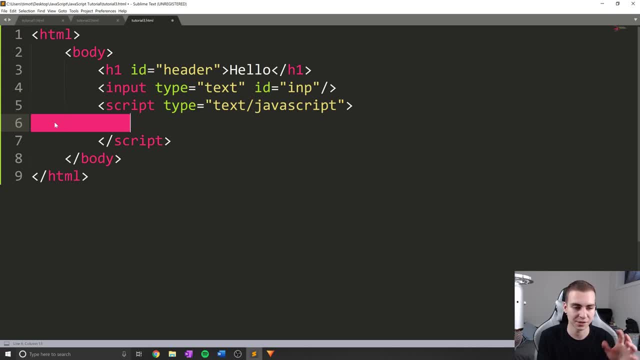 saying Java, but I really mean JavaScript, just because I do program in Java, So sometimes I mix them up. But anyways, the way that you define a variable in JavaScript is using the var keyword. Now, the first step when you're using a variable, we're going to make one, is to declare it, And that's what this statement. 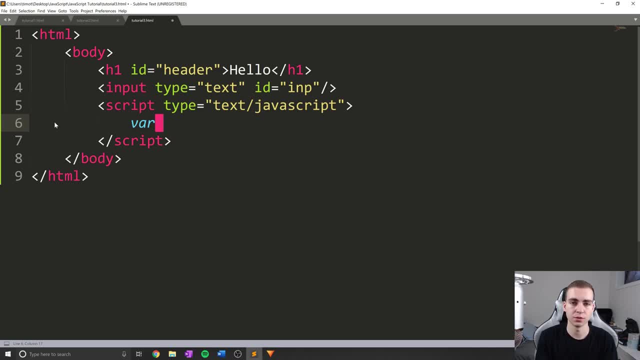 is going to be here declaring, creating, defining- those are kind of the words we use to say that. So here, what I'm going to do is I'm going to create a variable and I'm going to give it a name of x, So I'm gonna say var x And I'm going to use what I call. 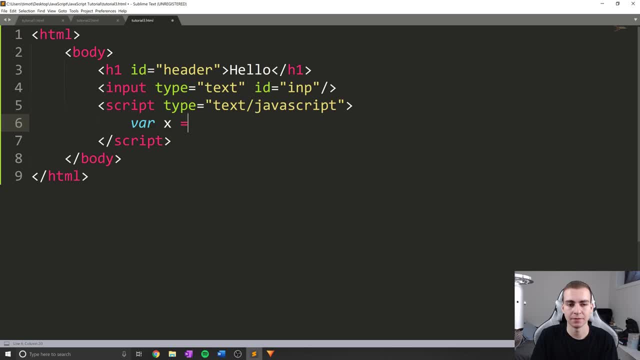 the assignment operator, which is an equal sign to assign a value to the variable x. So in this case I'm going to put six. now I'm going to put my semi colon to denote that we're ending this line, this operation And what I've done here is simply defined a variable. 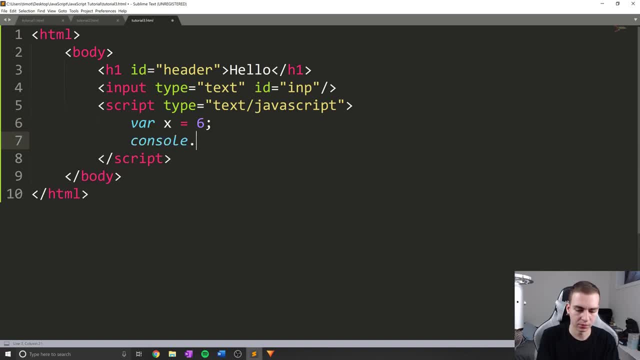 x, Which is equal to six. Now I'm going to show you, and I'll just do this here And you guys can guess what's going to happen, What happens when I do console dot log x. So if I run my 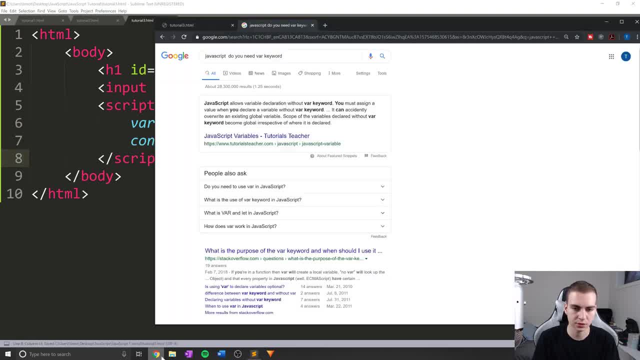 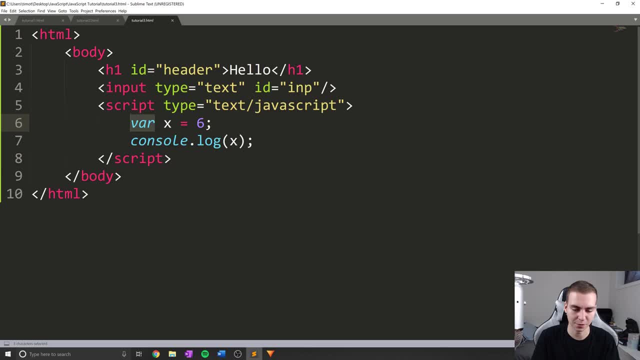 web page and I do console dot log x. what am I going to get? Well, before I tell you, let's run this And you guys can have a guess here. So there we go And notice I was looking up if you need to even use this before because I totally forgot. But anyways, we get six. 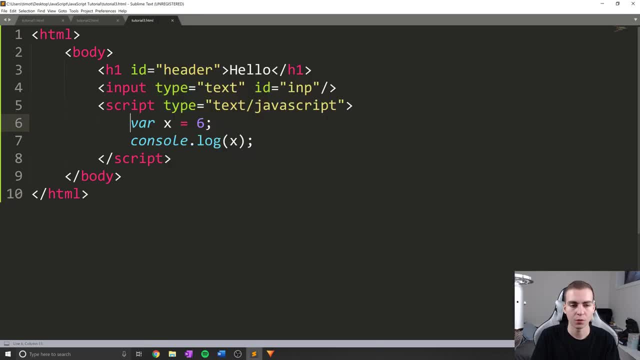 printing out to the screen. So how did that work? Well, the variable named x Stores the value six, And when I gain access to the variable x, when I type x here, it looks for the value of x, which in this case is six. kind of subsidence: we go six there. 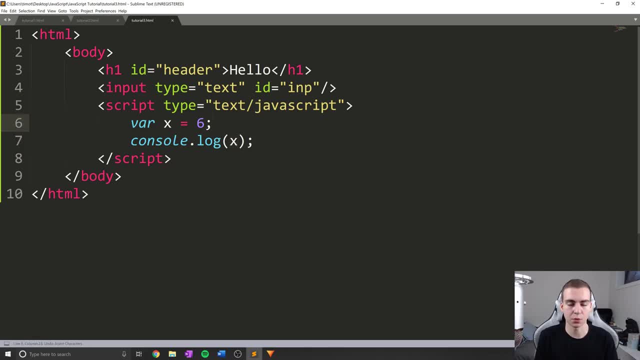 And then it prints that out to the screen. And this is the very fundamental, basic way that variables work. There's some name, some kind of pointer almost to an object, And when we access that name, it gives us the value that's stored inside of it. So, just like you, 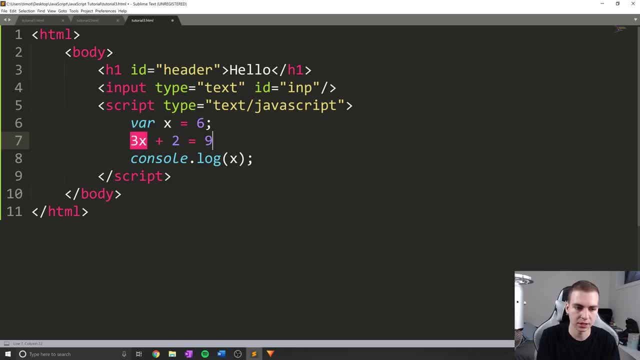 know when you have in math and you say like three x plus two equals nine, whatever you want to sum value like x equals nine. whatever you want to sum value like x equals nine. whatever you want to sum value like that x is a variable and it has some value. you 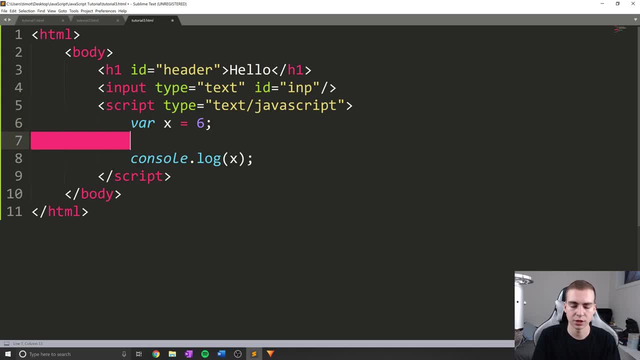 need to determine the value of it. So a little bit different in programming, because we just typically set up variables that are going to hold some information. we modify them and change them, But that's the basic concept behind a variable: some name that points to. 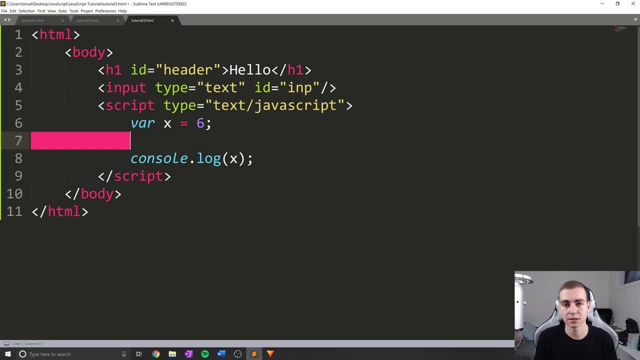 some value holds some value. when we access that name, we can simultaneously access that value. Now let's talk about changing variables. So here we've defined a variable called x equals six. But what if I want to change this variable to be the value nine? Well, since 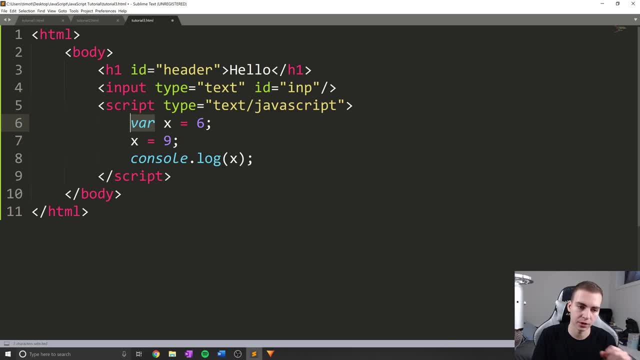 I've already defined my variable by putting this var keyword. here all I need to do is simply say x equals nine, And now, if I log x, notice that our value changes to not. So that's how easy it is to change the values. Now I want to talk about some rules when we do deal with variables and kind of. 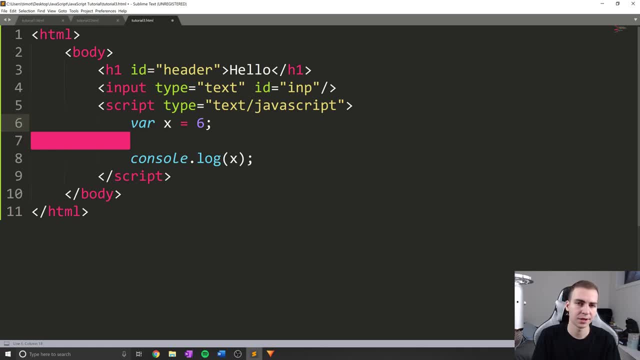 how we name them appropriately. So, typically and for right now, there's a lot of different ways to define variables. we're going to stick with this var keyword, but we'll talk about some others later And we need to define a name after we put var. that's going to be whatever. we're going to. 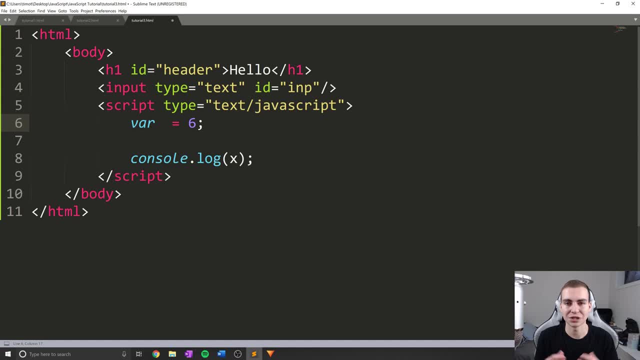 store. Now, usually we need this variable name to be meaningful. it needs to store something that makes sense, And the reason for this is when we look back at our program later, we're going to see all these different variables, all these different names. we're gonna have no idea what anything. 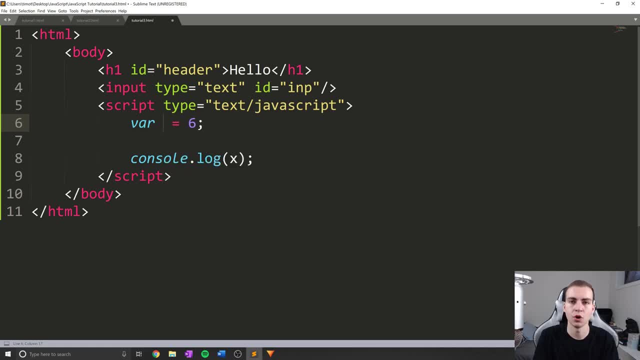 means if we kept naming them like t, z, C. we don't know what those variables mean, So we typically name them something that makes sense for what the value they're going to store. So let's change this up a bit And let's say: actually I want to create a variable that's going to store 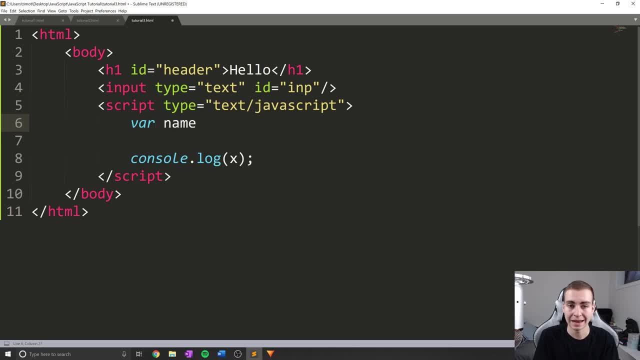 my name. Well, what I would do is I would say variable name, which is going to be the name of my variable, but coincidentally, actually the value name is equal to, in this case, Tim. Now quick quiz for you: What data type is Tim? Well, Tim is a string. So what I've done here is to find 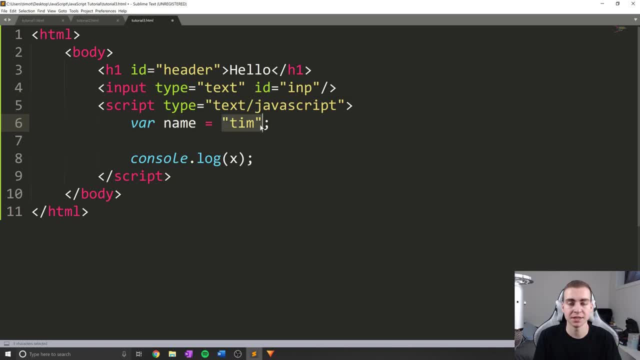 a variable called name, that storing the value Tim, which is of type string. So these variables can store, obviously, all those different things, But it's important we know these different types because the type of variable will allow us to do different things with us, different things with it. 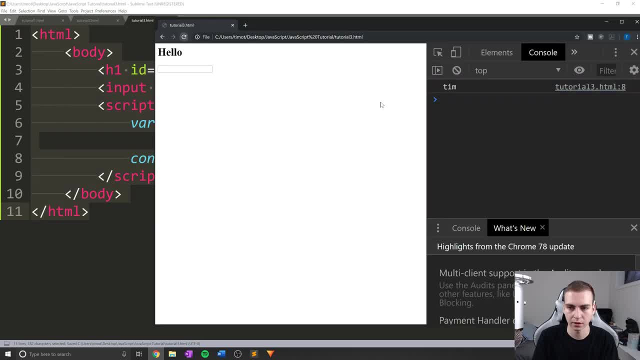 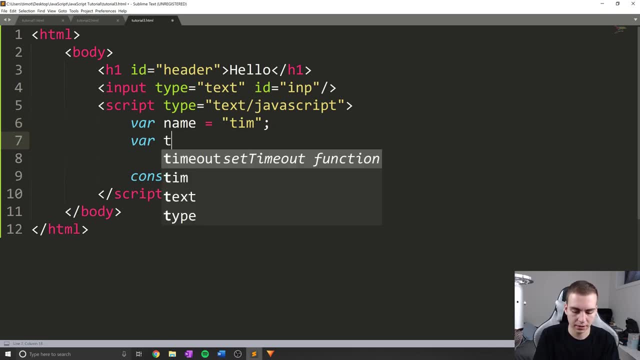 sorry. So let's print out name and just make sure this is working. There we go. we got Tim. Awesome, Good to go, Okay. so let's create some other kind of variables. So let's say: var t- hello, equals five. Now this actually has an issue with the variable that I've created here. 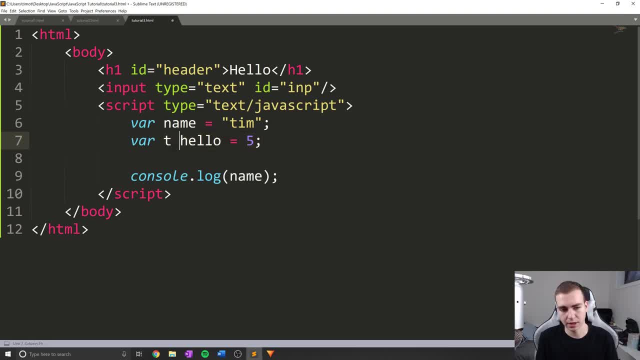 And this is what I want to get into. my next point, And how do we make valid variable names? Well, there's a few rules when we define a variable, one of which is that we cannot include any spaces in our variable name. we want to do something that looks like a space. what we are allowed to do is 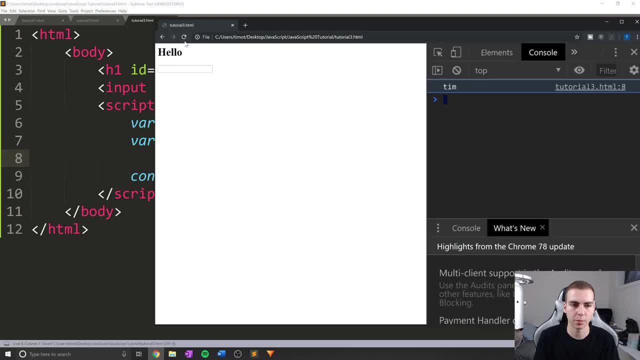 underscores. But if I do a space watch, what's going to happen when I run my program. We're going to get an error in our console. Now why did that happen? Well, because it's saying there's an unexpected identifier. Now, this is what I want you guys to do, Whenever you know. 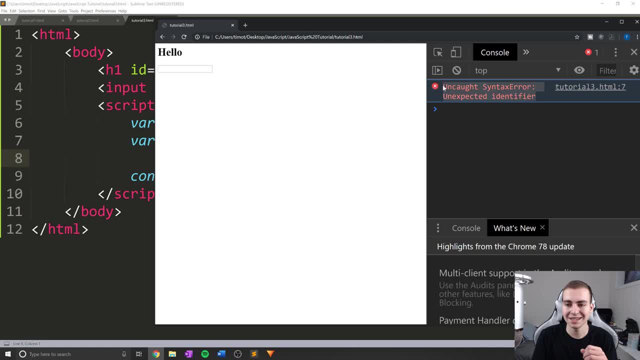 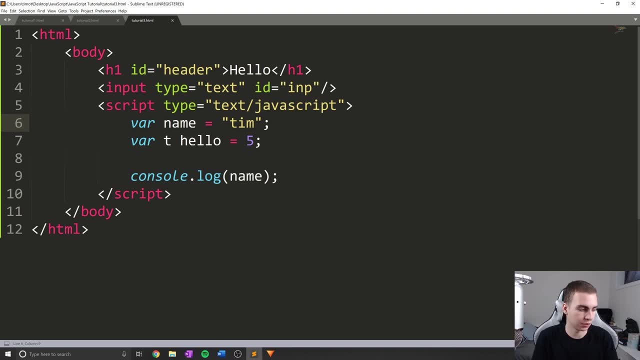 you make a mistake, something happens. open up your console and see if you have any errors here. If you do, you can Google search them. you can figure out what the issue is And then hopefully that will help you kind of fix your problem. But those error messages have meaningful information. 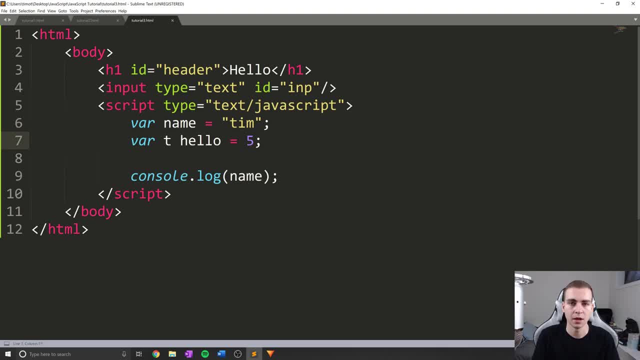 in them, So try to read through them. you probably won't understand what they mean immediately, But if you Google, search them. hopefully the next time you run into that error message you're going to get an error in our console, And then you're going to get an error in our console. 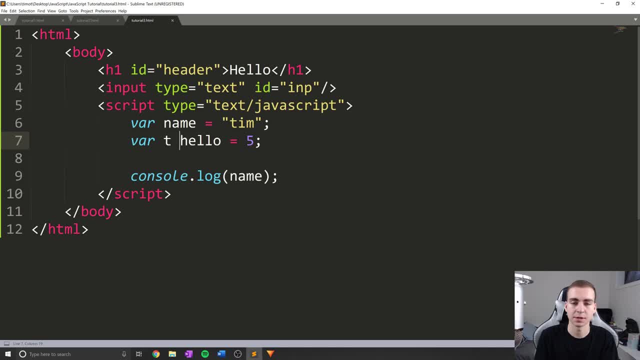 You might understand where you might have gone wrong. So, anyways, in this case that's because our variable name is named incorrectly, So what I need to do is either add an underscore or change it so that it has the rules applied to it. Now, some more rules for variables are that you're? 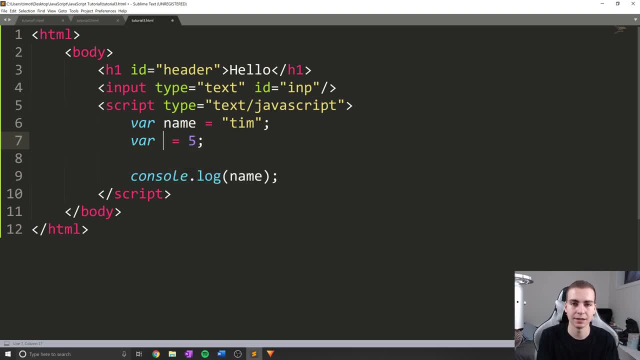 allowed to use any characters, So any characters on your keyboard that are letters or digits. that means I cannot use, like brackets and you know, all these other symbols inside a variable name. I need to use only letters and numbers And those letters can be uppercase. 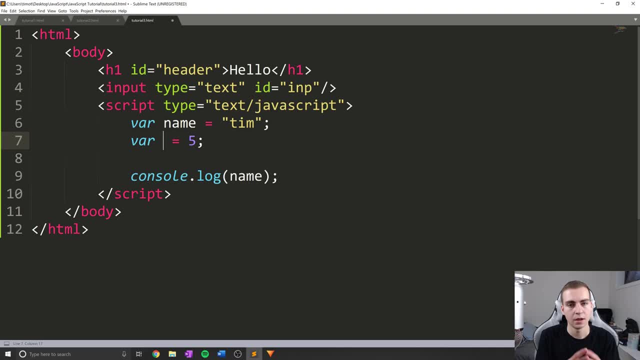 lowercase. that doesn't matter. Obviously, you can do the numbers how you'd like. Another rule that applies to variables is you cannot start your variable with a number, So I can't do something like five, hello, and you can see we're getting highlighted like this: there's an error here. 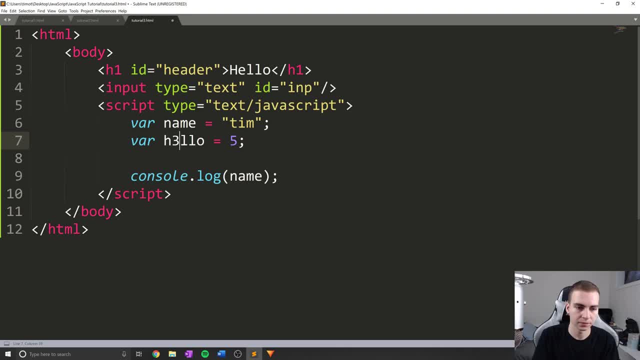 what we need to do is we do something like hello five. we could do, you know, h3, lo, that's fine, we just can't start with a number. So those are kind of our basic variable names. Now, if we want to do a variable that you know says has like three or four words combined into it, 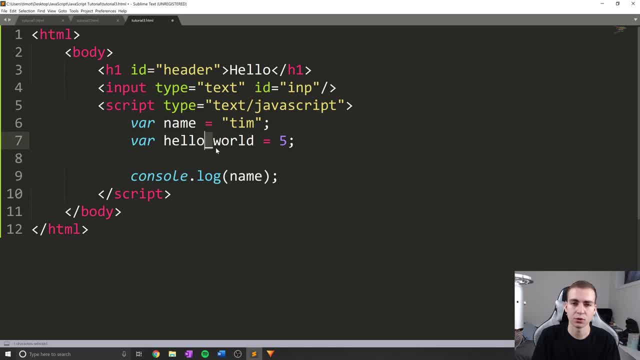 say, for example, Hello world. it makes sense to typically set separate your words with an underscore or to do some camel case like this: So hello, and then capital on the next words. that's easier to read. So I just figured I mentioned. 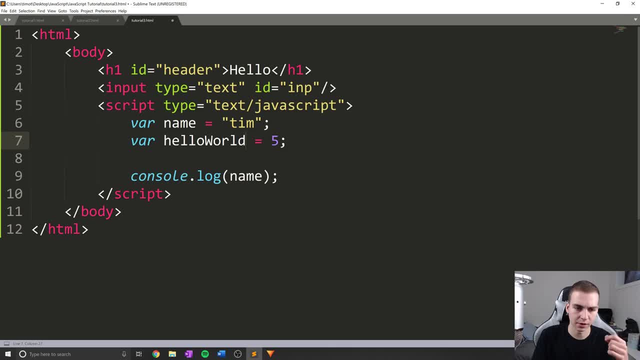 that to you guys. Okay, so there we go. we have our variable name. we have a variable Hello world. Now, what I'm going to do is do something you guys probably haven't seen before, which is actually set the value of Hello world to be equal to name. Well, what is this going? 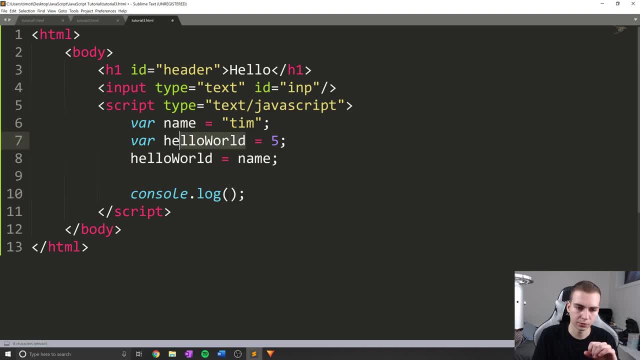 to do? Well, what we're going to do is we're going to look at Hello world. we're gonna say: okay, this is equal to five. what we're going to do now is change the value. we're going to change it to name. 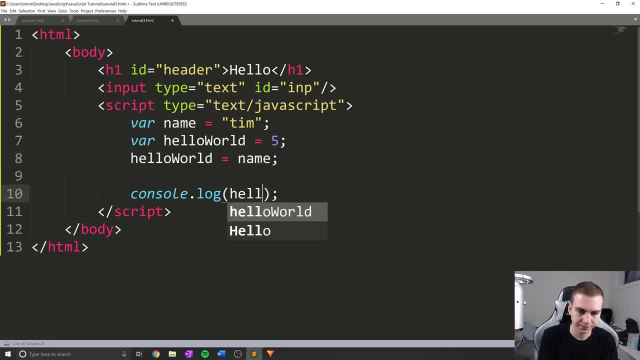 What is name store? name store is the value Tim. So that means if I print out Hello world like this, we get the value Tim. So that is totally valid. we can definitely do that. we can set a variable to equal another variable And that is totally okay And notice that. 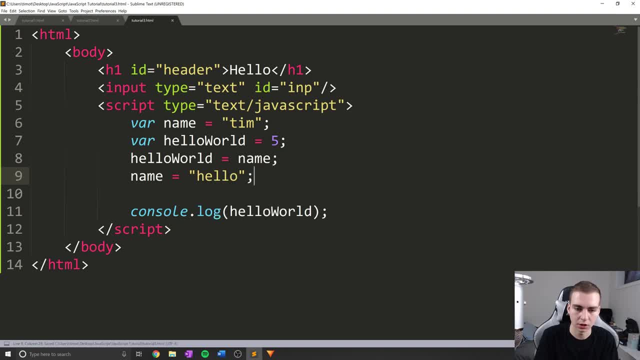 if I actually change the value of name, so I say name equals Hello, like this. let's see what happens. Nothing changes And that's what I want you to notice, Because I defined Hello world equals name Before I change the value of name. Hello world is still going to have Tim as its value. 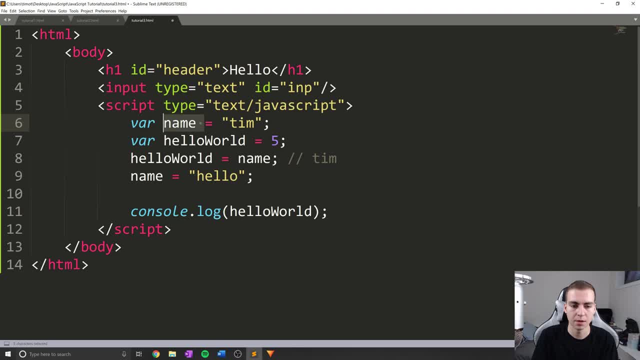 And that's because when I defined it here, Tim was the value of name, but then I changed name after here. So let's actually console dot, log name like this and show you what that is. So we'll do it before like this. So we'll do it right when we define it then.